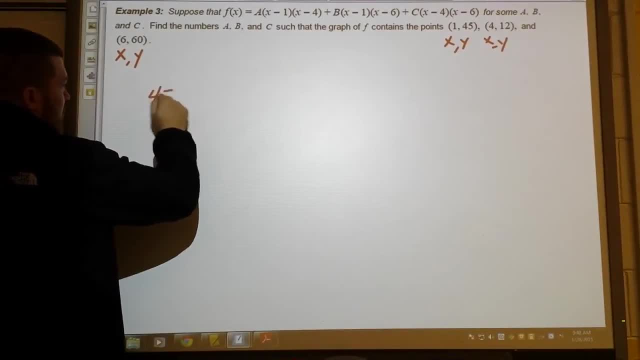 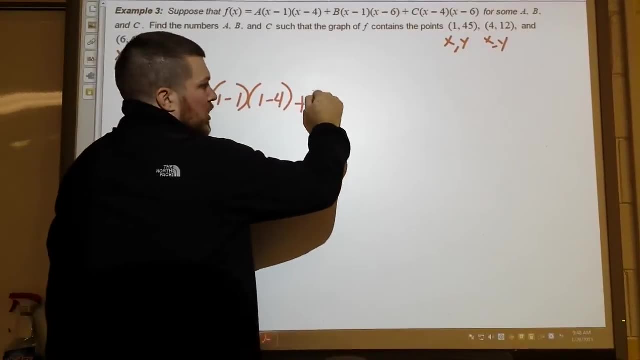 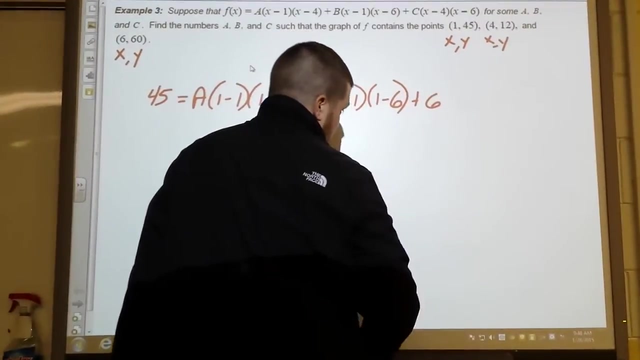 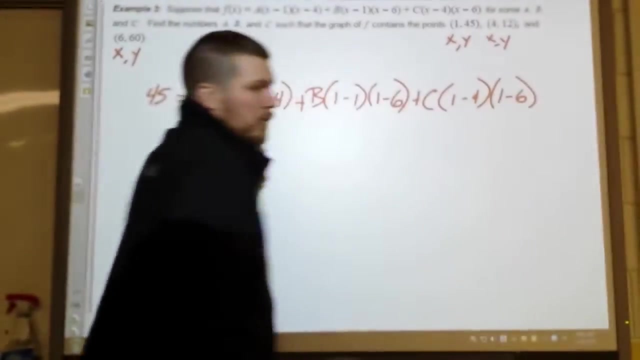 I'm going to plug in a 45. So I have: 45 is equal to a times 1 minus 1 times 1 minus 4 plus b times 1 minus 1 times 1 minus 6 plus c times 1 minus 4 times 1 minus 6.. Now I want to clean this up as much as possible, So in 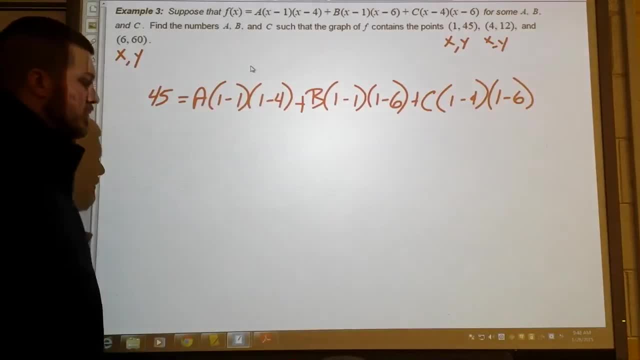 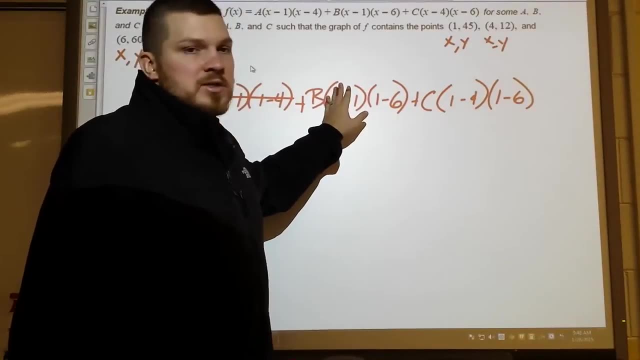 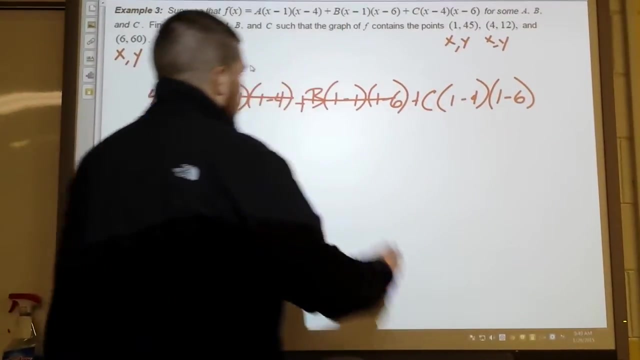 my first term. 1 minus 1 is 0. Anything times 0 cancels out, So this piece is gone. Same thing happens in the second term. 1 minus 1 is 0. So this piece cancels out and is gone. The only piece that's remaining is my third term, So I have 1 minus 4, which is 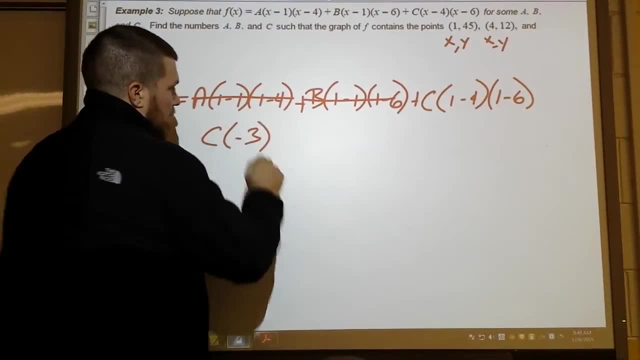 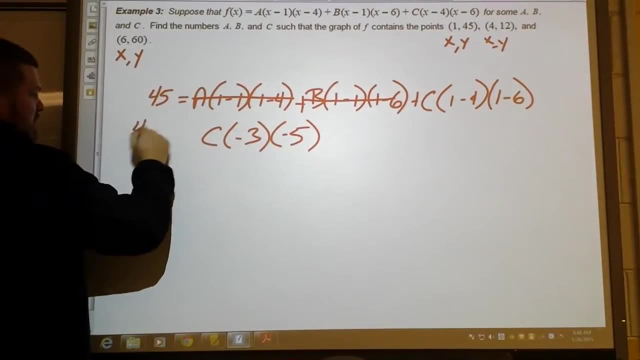 negative, 3.. So c times negative, 3.. 1 minus 6,, which is negative, 5. And 45 just falls down. Now I can clean this up. Negative 3 times negative, 5 is positive. So I can clean this up as much as. 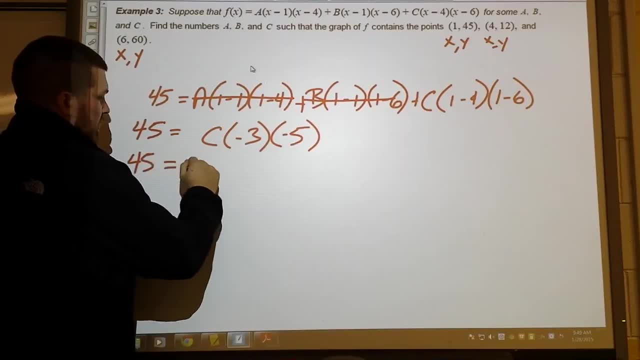 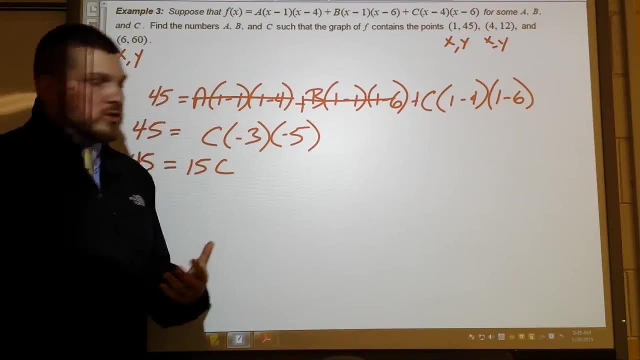 I want. So I have 15.. So I have 45 is equal to 15c. Now this is multiplication 15 times c. To undo multiplication we need to divide by 15 on both sides. Doing that, I find that c is equal. 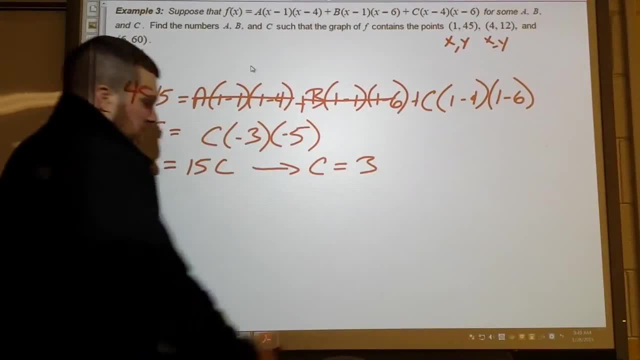 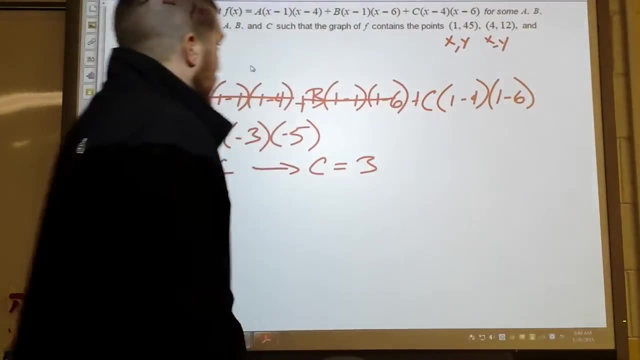 to 3.. Great, So we're done with that first point. Now I want to do the same idea with the second point. Everywhere I see an x plug in a 4.. Everywhere I see a y plug in a 12. So I have 12. 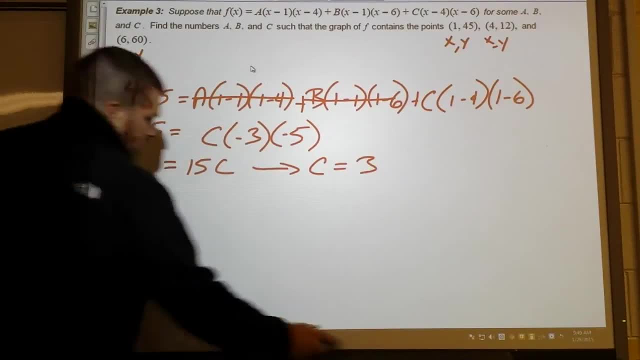 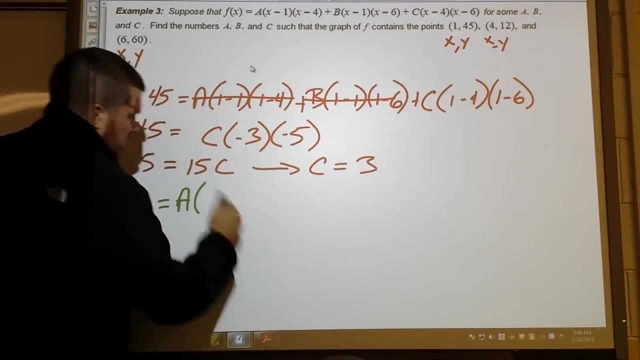 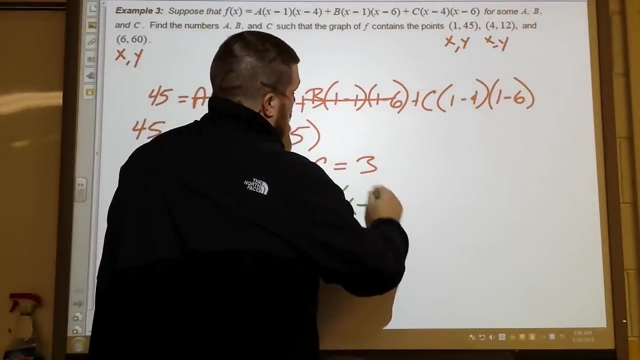 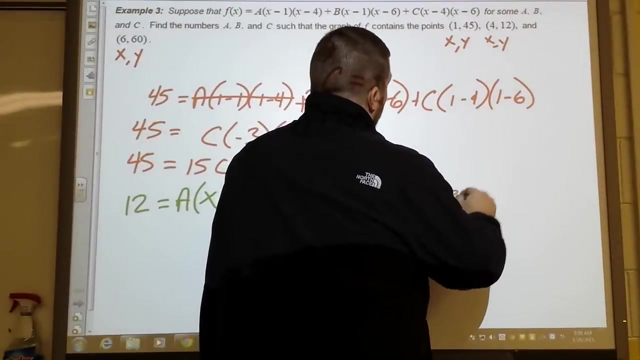 is equal to 15.. A times x minus 1 times x minus 4, plus b times x minus 1 times x minus 6.. And since we know what c is, I can now plug that in. So plus 3 times x minus 4, x minus 6.. And again, everywhere I see. 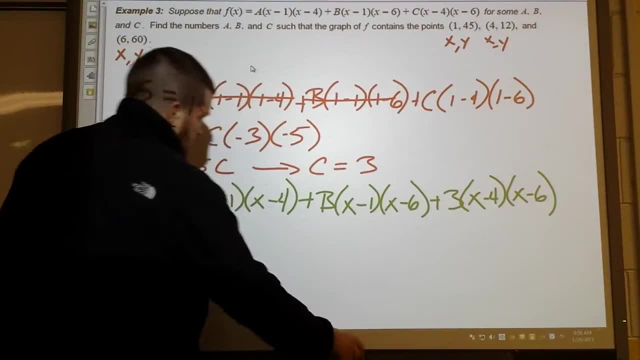 an x. I'm going to plug that in. So I'm going to plug that in. So I'm going to plug that in. So I'm going to plug in a 4, which I honestly should have done earlier, but I forgot That's. 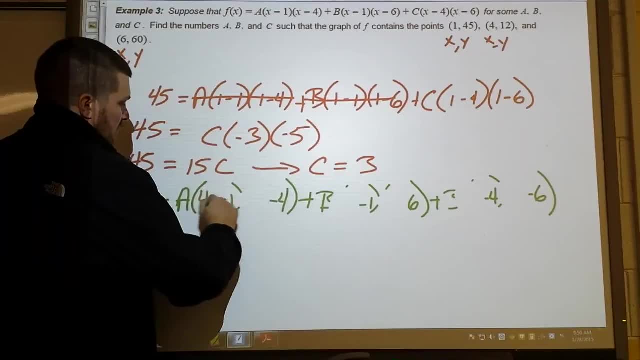 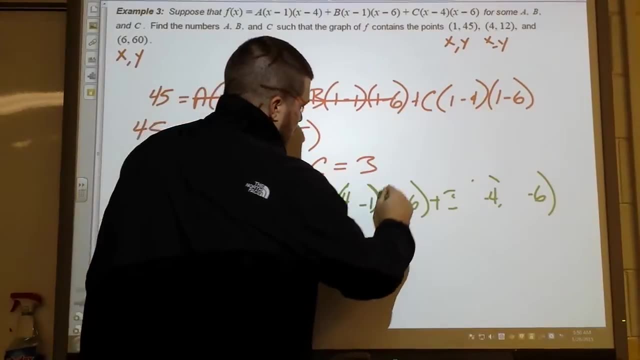 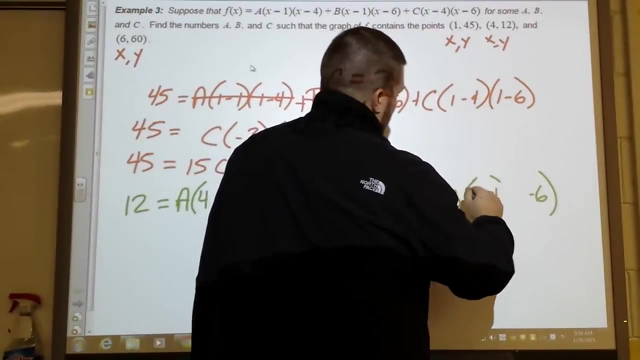 okay, So just go back and fix it. So I have 4 minus 1 times 4 minus 4 plus b times 4 minus 1 times 4 minus 6 plus 3, which was our c times 4 minus 4 times 4 minus 6.. 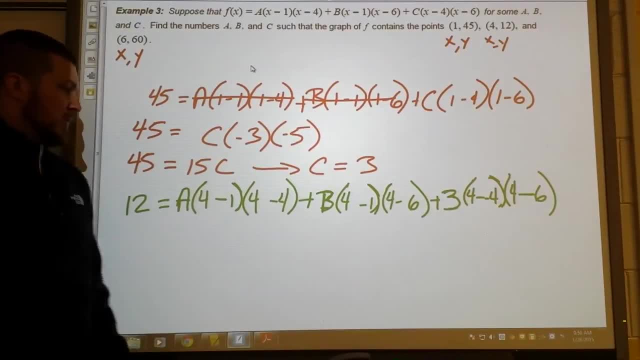 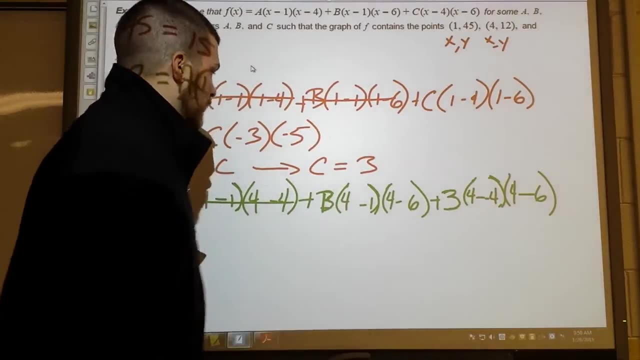 Okay Now what I want to do is just simplify as much as possible. In my first term, 4 minus 4 is 0. So my first term is going to cancel out. In my second term, 4 minus 1 is 3.. So I have 12 is. 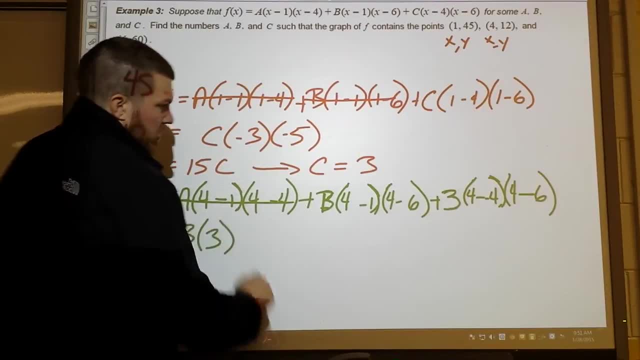 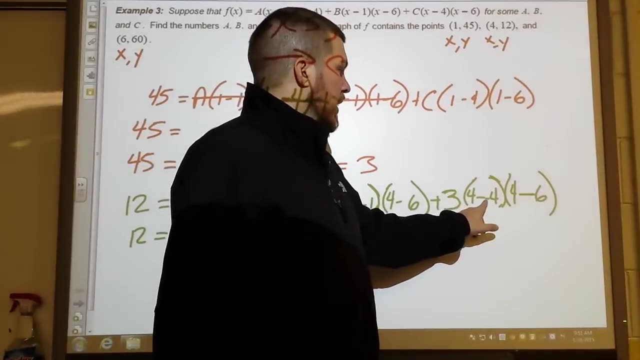 equal to b times 3.. 4 minus 6 is positive 2.. Okay, And in my third term, 4 minus 4 is 0.. So my third term is going to cancel out. So this is all I have left, using my second point. So I'm going to. 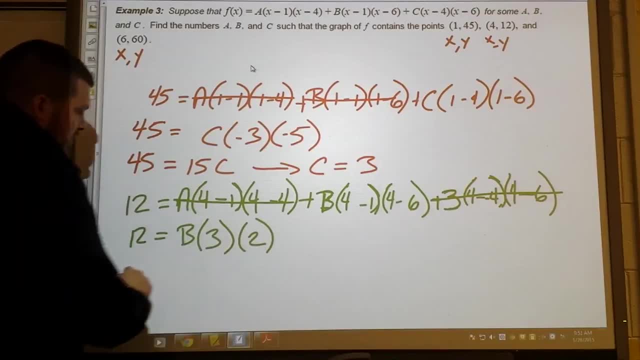 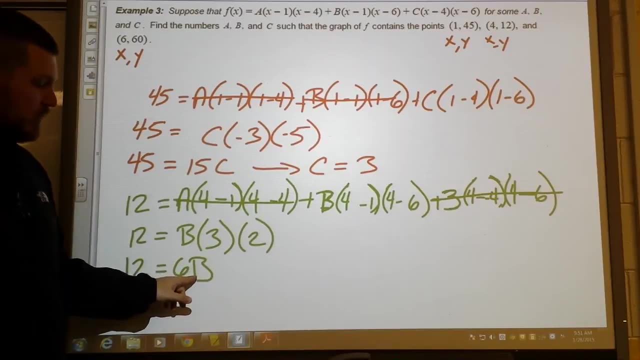 clean this up and figure out what b is. 3 times 2 is 6.. So I have: 12 is equal to 6b And again, this is multiplication. So to undo multiplication we need to divide on both sides So we find out. 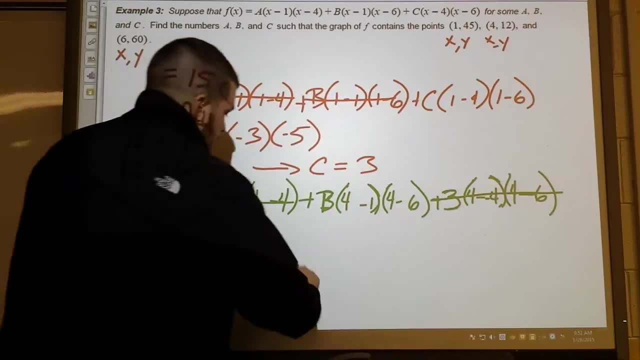 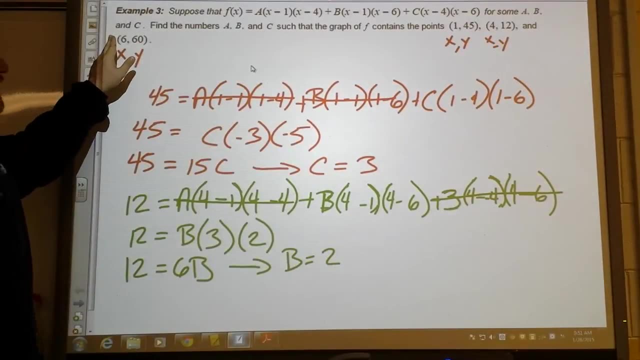 by dividing by 6 on both sides, that b is equal to 2.. Okay, And then, finally, we only have one point left: 6 comma 60. So everywhere I see an x, I'm going to put in a 6. Everywhere I see a y, I'm. 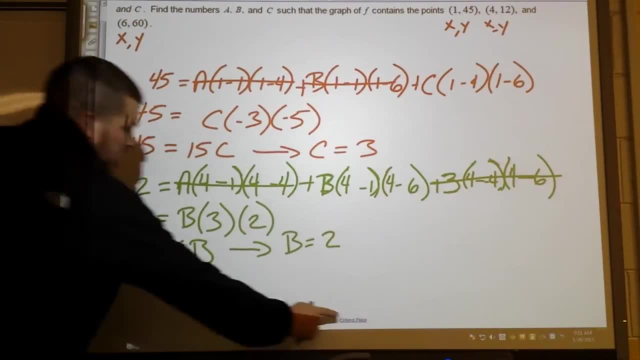 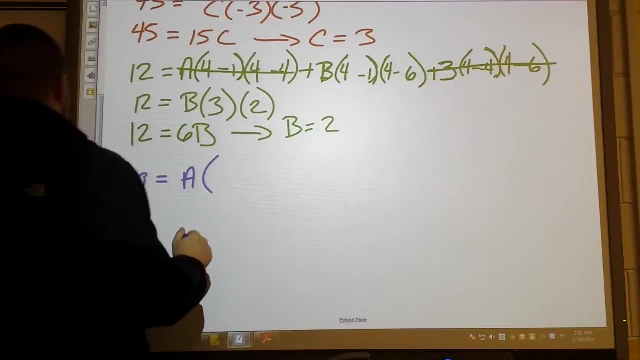 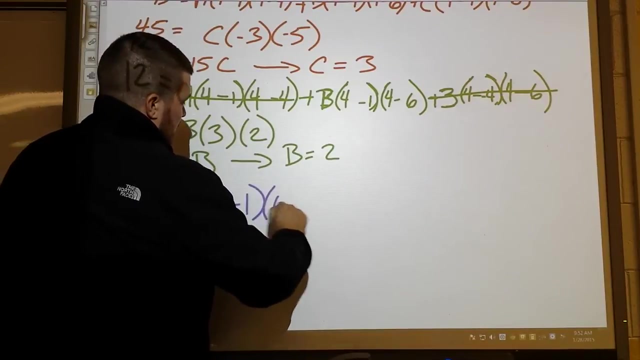 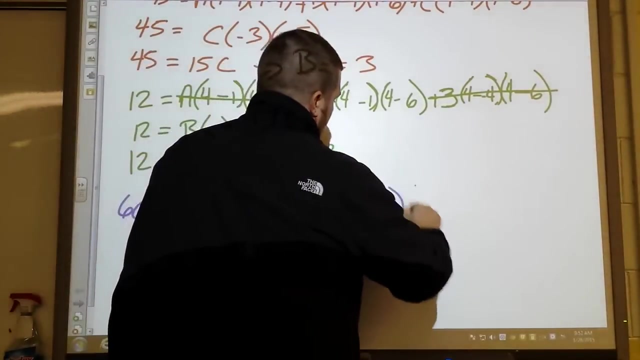 going to put in a 60.. So just repeat the same process I have: 60 is equal to a times 6 comma. everywhere I see an x. I'm going to put in a 6.. So 6 minus 1 times 6 minus 4.. Now we know what b is, so we can plug that in. So plus 2 times 6 minus 1 times 6. 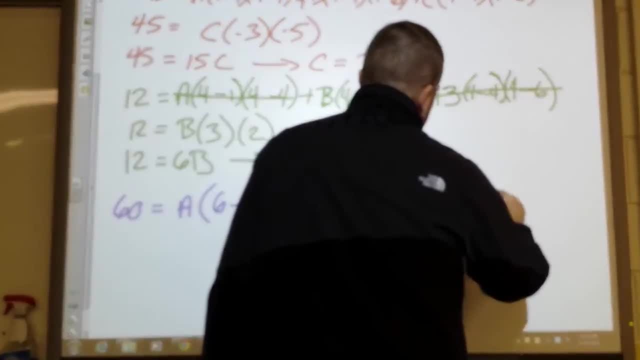 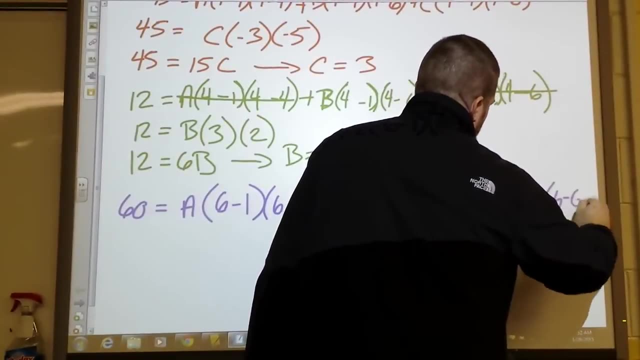 minus 6.. And again we knew that c is now 3.. So 3 times 6 minus 4.. And again 6 minus 6.. So we want to clean this up as much as possible And we'll find our last. 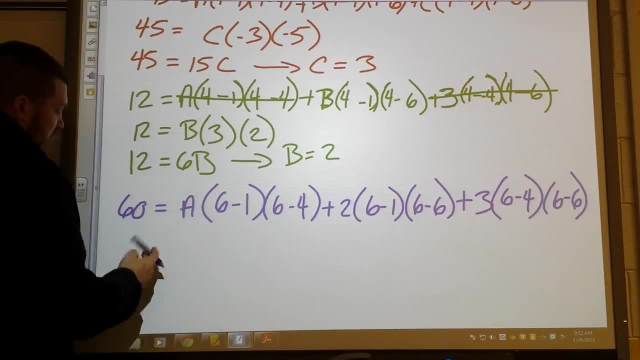 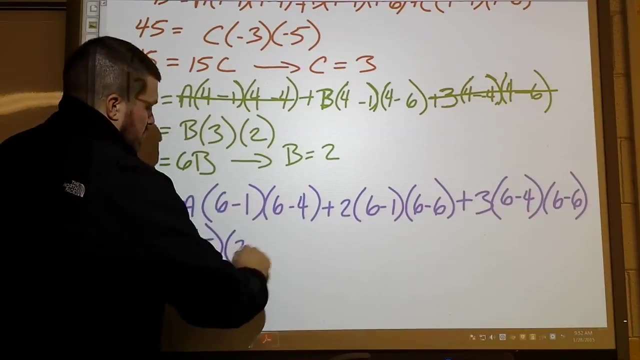 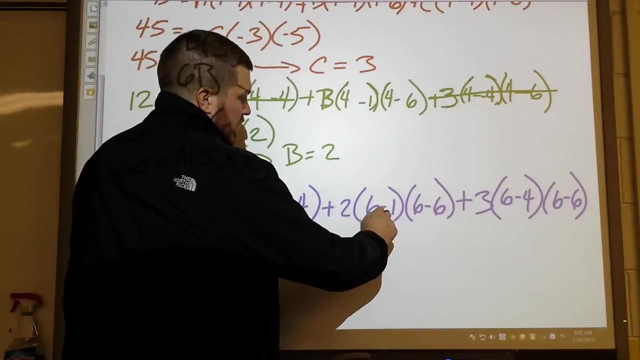 coefficient. So in my first term 6 minus 1 is 5.. So I have: 60 is equal to a times 5.. 6 minus 4 is positive 2.. Okay, And in here my second term: 6 minus 1 is 5.. But 6 minus 6 is 0. So my second.